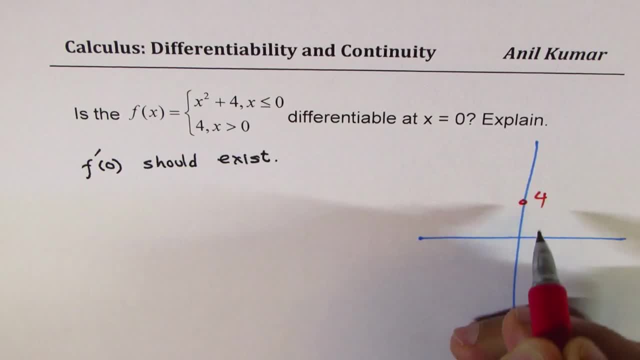 unity. So we know when x is less than equal to 0, it's a parabola which has been translated for units up, So 4 units up. This is the point at 4.. On the left side is going to be a parabola like: 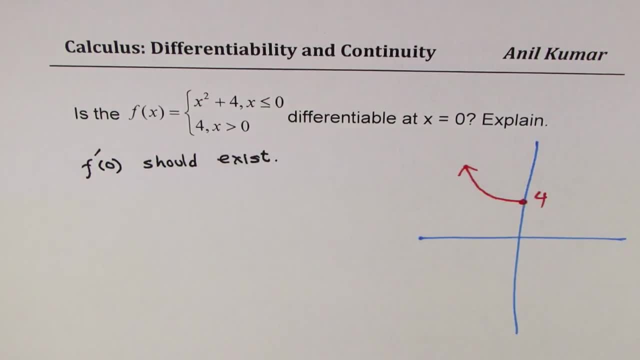 this right On the right side of y-axis. it is a constant function, 4, right. So it is a straight horizontal line. So it is continuous at x equals to 0.. However, we have to find whether it is. 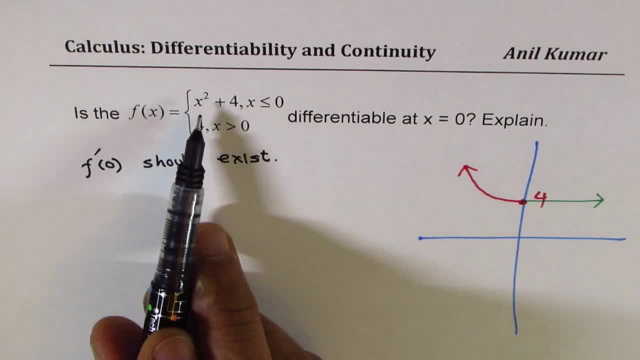 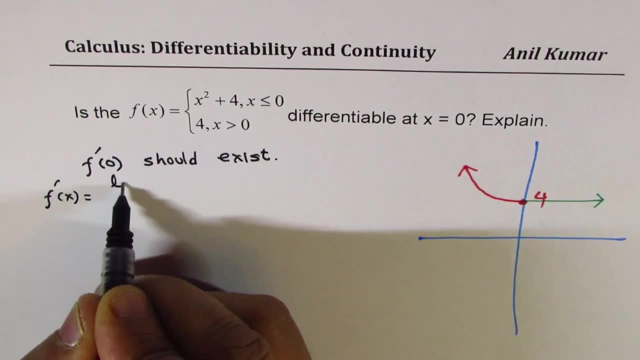 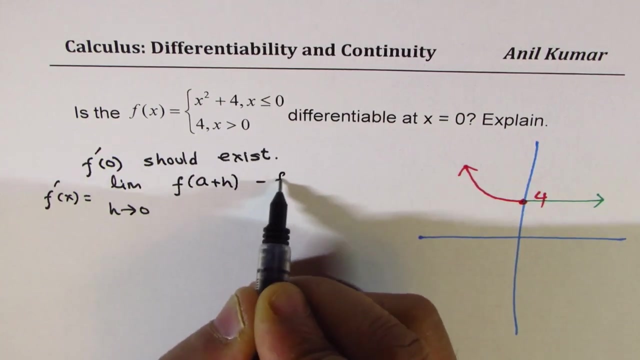 differentiable or not. So that means we'll treat it in two different parts And with the definition we know, f dash x is equal to the limit. h approaches 0 for f of a plus h minus f of a over h. So that is. 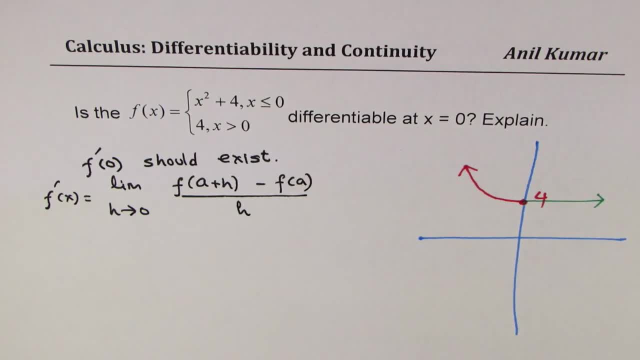 the fundamental definition for finding the derivative at a particular point. Now, in our case, a is equal to 0, right, When we say x equals to 0, the value for this value of a is 0. So we'll find both the limits, one from the left side, So left side when x is less than equal to 0. At that time, 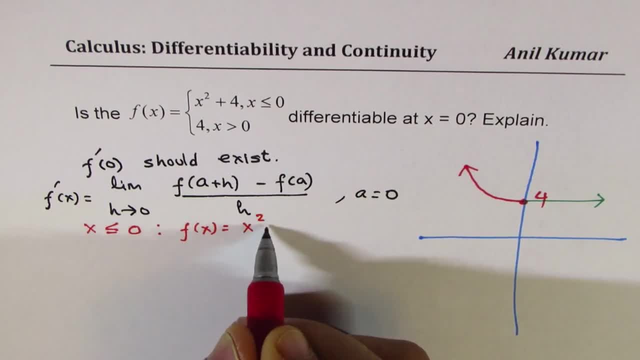 f of x is equal to x squared plus 4, correct? So we'll find this left side limit And we'll also find the limit when x is greater than 0. And in that case we know f of x is equal to a constant function 4.. Is that? 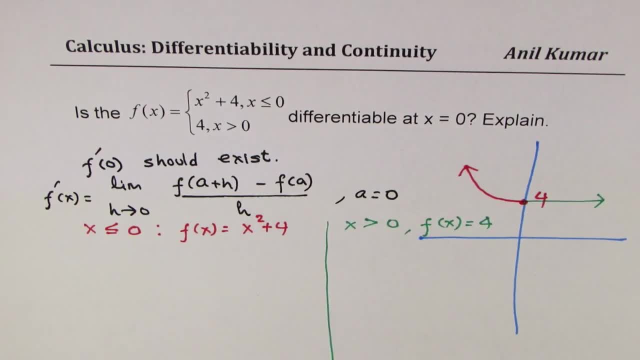 clear: A is equal to 0. So the general expression for the derivative will be f dash. x equals to limit. Now, when we are talking about this function, h approaches 0, it is going to be x plus h, whole square plus 4. so that is a plus h. you can say right, minus. 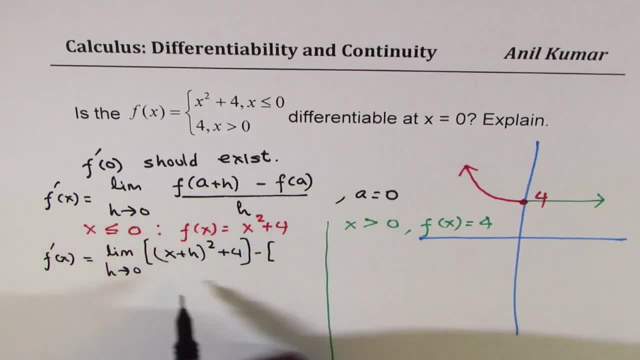 f of a will substitute a equals to 0. later will be x square plus 4 right divided by a. so that is the general expression. now, in this expression i am substituting the value x equals to a, which is 0, right. so if, if i am finding at 0, x becomes 0, is that clear? so if i write 0 here, 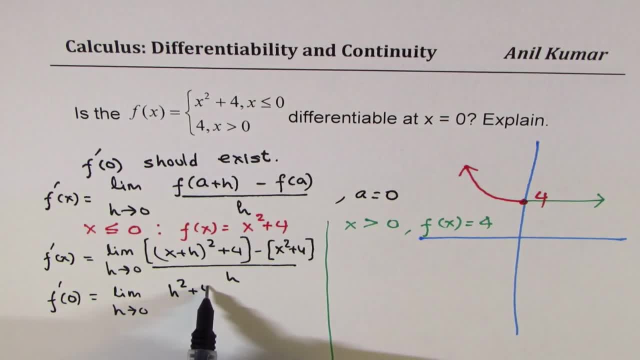 i get h square plus 4, x is equals to 0. right and on the right side, what i get is x is 0. i get minus 4 over h. is that clear? so that gives you limit h approaches 0 of h. square over h, which is limit. h approaches 0 of h, which is 0. perfect. so that is how, from the 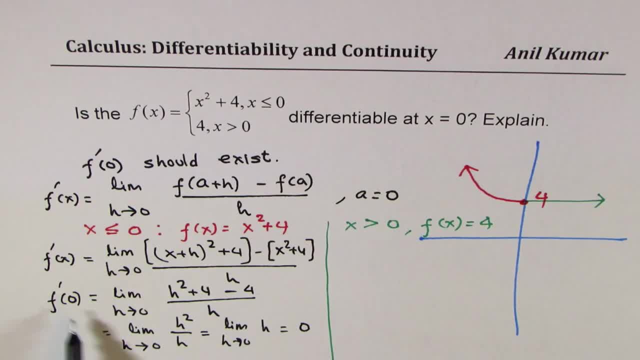 left side, you find that the derivative is 0. now let's do the same on the right side. so in that case, what do we get? so the limit h approaches 0. now the function is 4, right, so so there is no x in. it's the both. if you take two points here, they are just four, right, so it is. 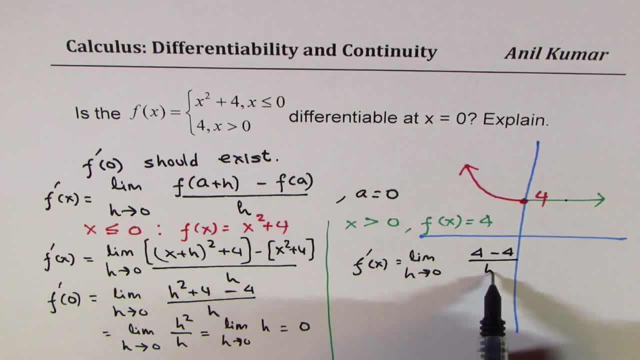 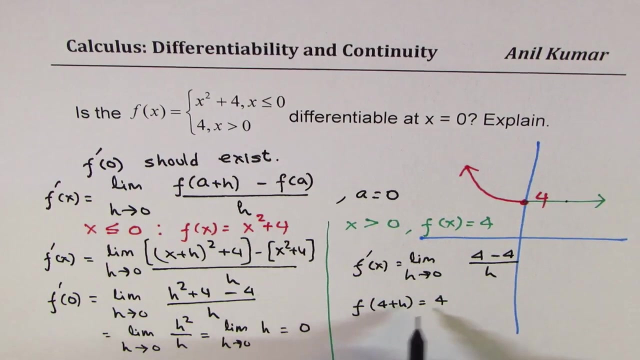 4 minus 4 over h. right, because in this case, as you can see, f of 4 plus h is also equal to 4, perfect, that is why. that is why this is constant. so i mean: so that is why this is constant, constant. so i mean 0 plus h is 4, i mean 0 plus h. if a is 0, it is at every place, it is 4, so this: 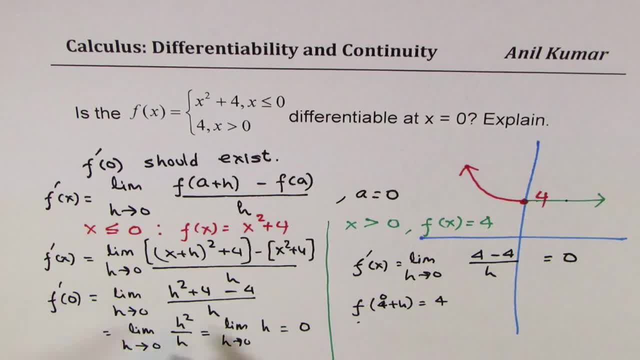 is equal to 0. now what we notice here is that both derivatives from both the sides are having the same slope. so horizontal line is the slope right. so we see that the horizontal line is slope at the point 0, 4, correct? so, since we see that the derivative exists, since we know